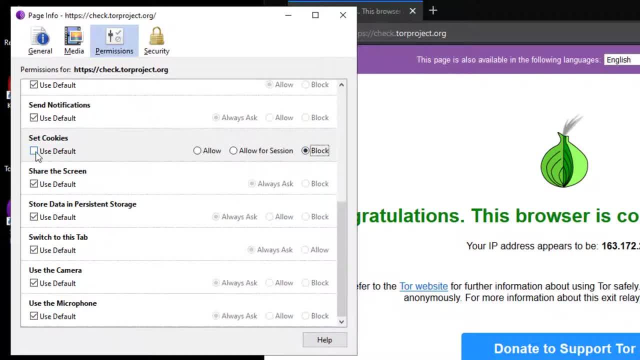 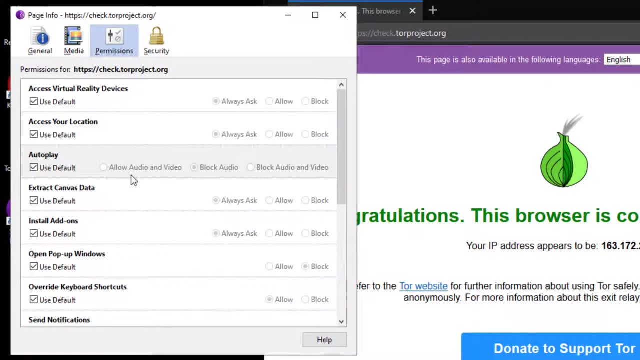 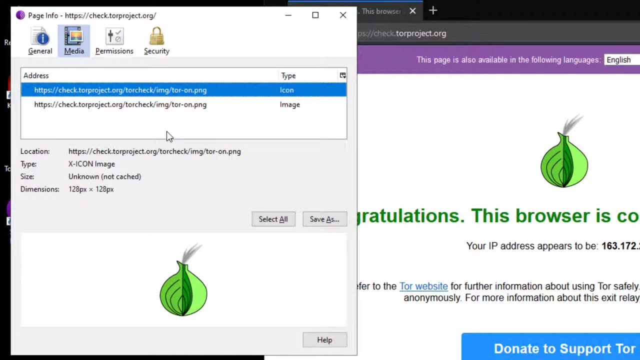 for your security, it would be much better to keep the settings here default, But of course you can change these permissions differently from the default, especially for the website you trust, whenever you need them. For the Media tab, you can obtain the information of the materials, such as pictures and videos. 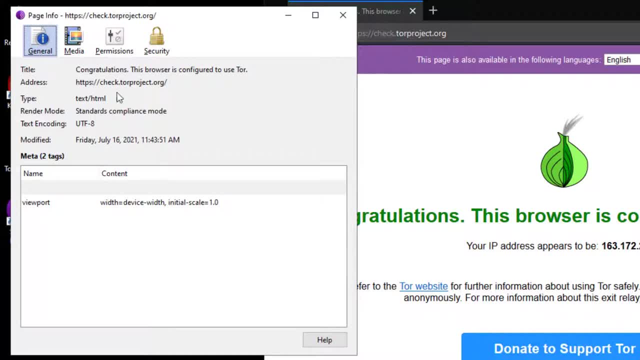 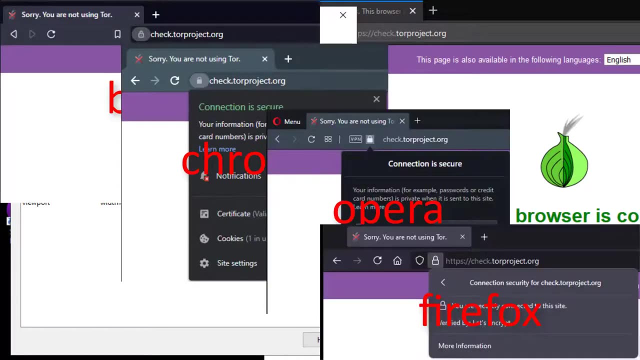 owned by website. In the General tab, you can obtain general information, such as the title and addresses of the website. I also want to remind you that this feature- the ability to get information about, certificate and manage site permissions- is not only available in Tor Browser. I just want to talk about 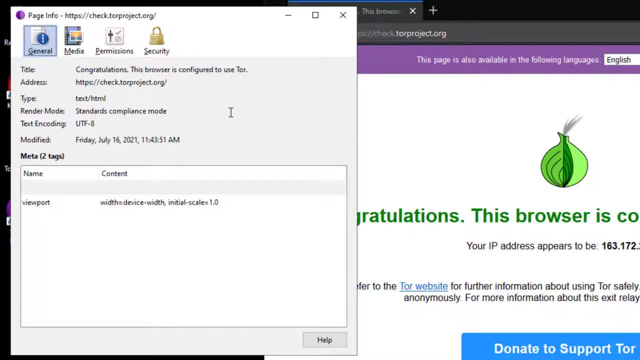 it. in case you don't know or don't care. if you know, Checking such information about the website you are visiting to and managing its permissions is a very good habit in terms of security. Even if you haven't paid attention to this until now, you have now learned that. 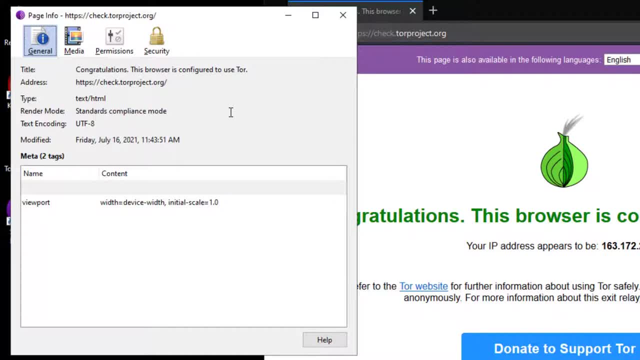 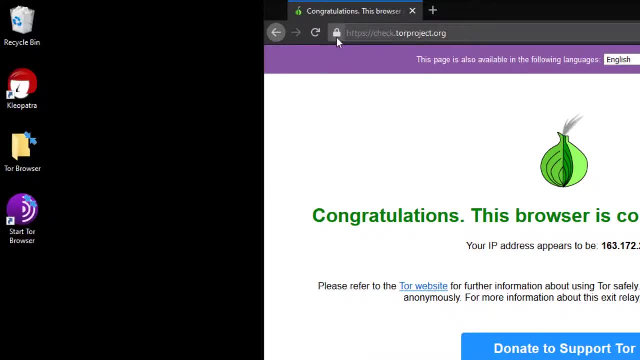 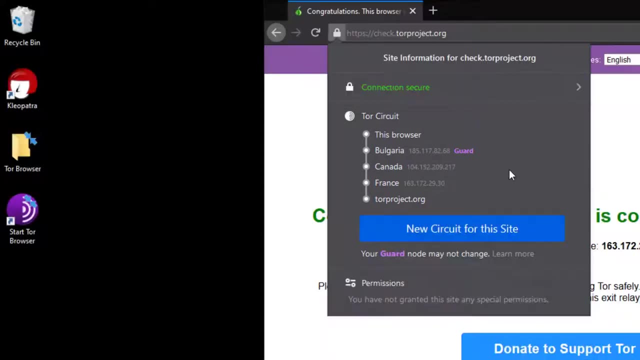 it is an important detail to pay attention to this part for your privacy. You know Tor Sources gives the information of the servers you are connected to Tor Network. As you can see, I am currently communicating with checktorprojectorg via this Tor Sourcet. Except for the first node in the Sourcet. the middle and exit node can be easily changed with the new Sourcet for this side button here. In addition, if you don't refresh manually, the Sourcet will automatically change itself every 10 minutes, except for the entry node. But why does the entry node stay the same despite the renewal? This is because the entry node in the Sourcet is selected as a guard. It is a fast and stable node that stays at the same for 2-3 months, as we have already mentioned, to protect against. 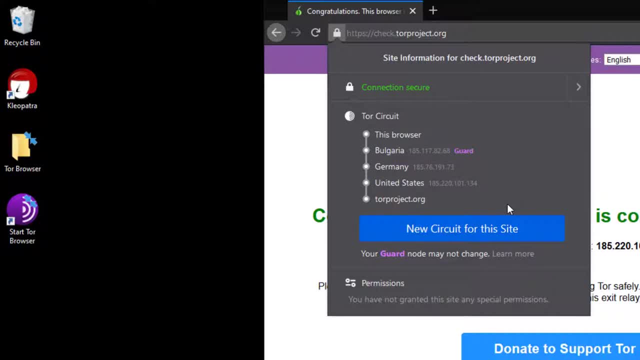 attacks that could compromise your anonymity. The entry node usually doesn't change for the 2-3 months, unless there is a server side issue. In exceptional cases, when your security is at stake or your server is not working properly, a security notification will be displayed So you will have access to your security. 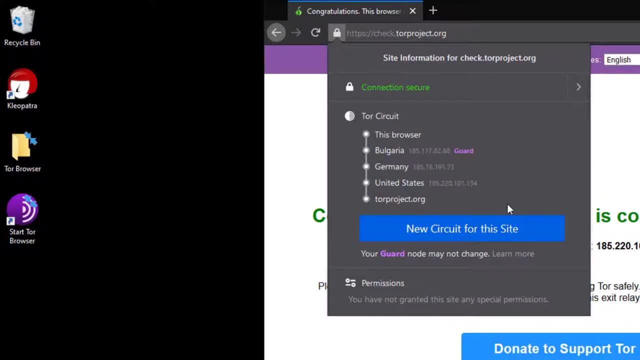 properly, you can witnesses its change automatically in short time. In short, the fact that the entry node doesn't change is the most effective security method that can be used now. protect against possible attacks on the Tor network. contrary to feeling of insecurity it creates in you For more technical, 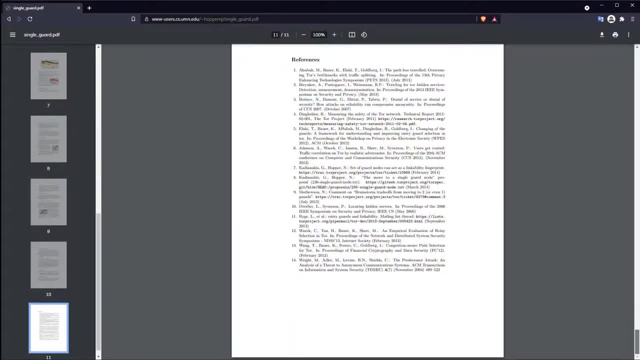 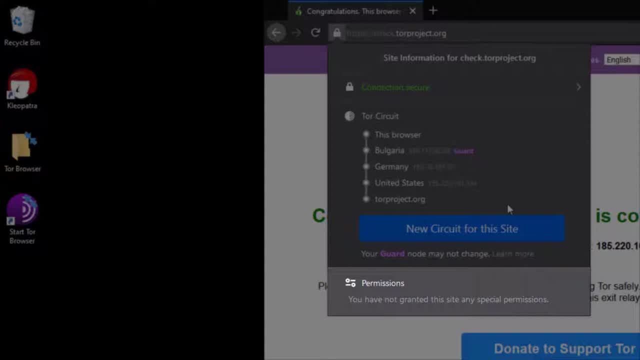 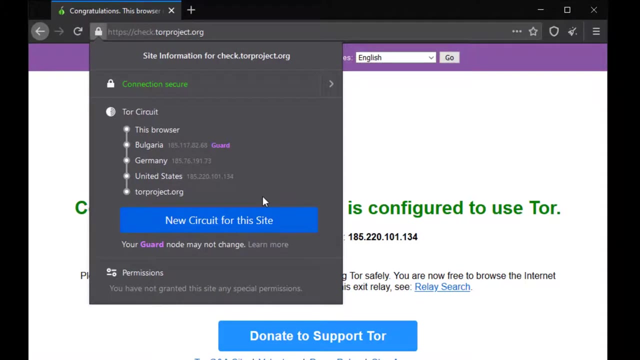 details. you can read the article published by University of Minnesota from the link at this: lecture resources. The permissions section under the Tor circuit shows the site specific permissions. I will comment the permission issues again. I was explain the settings in a moment. Now let's talk about the